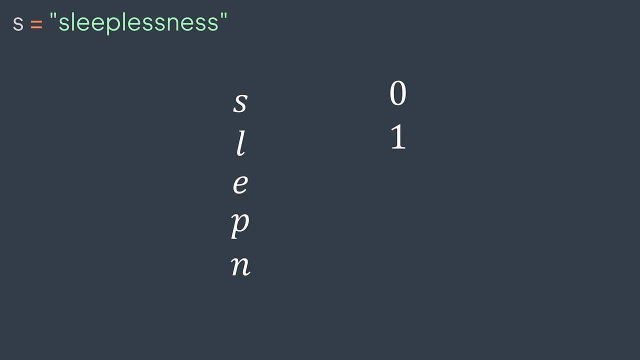 ones. We take the code zero, the code one. then we cannot have another code with one bit only. we move to two bits. We take the code 00, the code 01 and the code 10.. But how to assign them to our characters? Do we do it randomly? No, Our goal is to reduce. 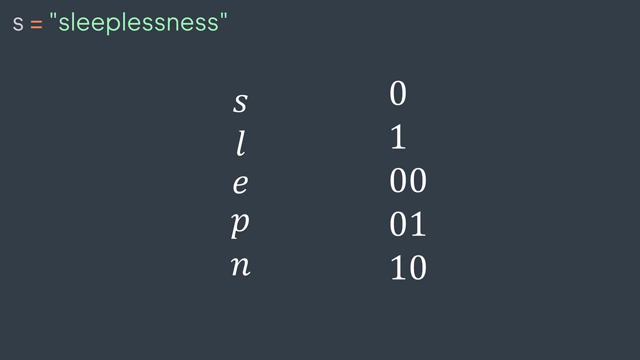 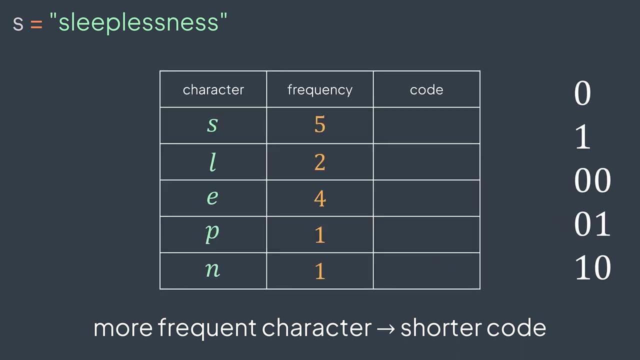 the total number of bits to represent the string. So clever thing to do is to give shorter codes for more frequent characters. Here, as has five occurrences, L has two occurrences, he has four, P has one and n has one. We saw them by frequency and we assign to them the code, sorted by length. Look at: 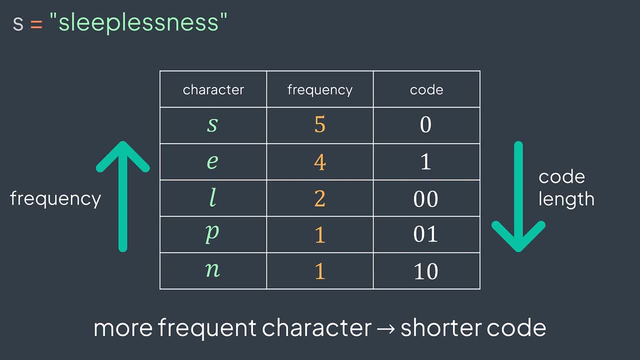 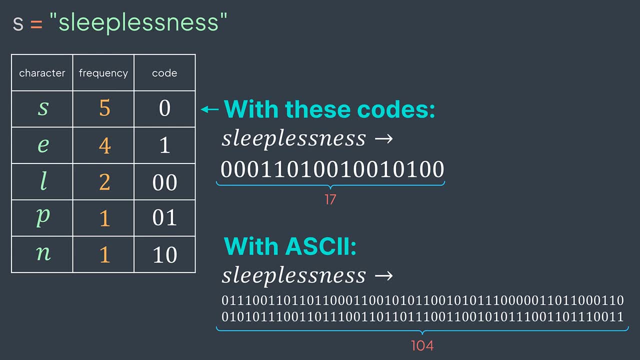 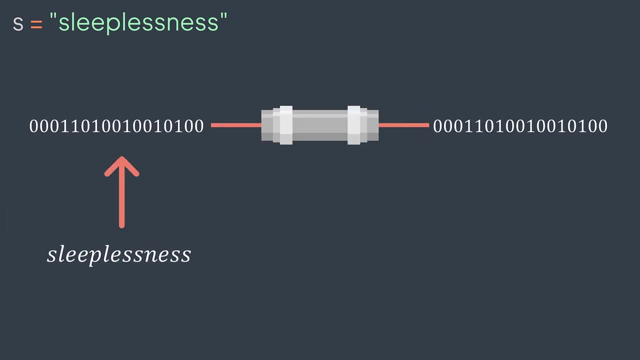 zero for s14 is 004 l014 P and one zero for n. Now if we replace each character by its code, we got a total length of 17 bits, way better than the 104 necessary bits. by using ASCII, We encode a message to sort or transfer it. 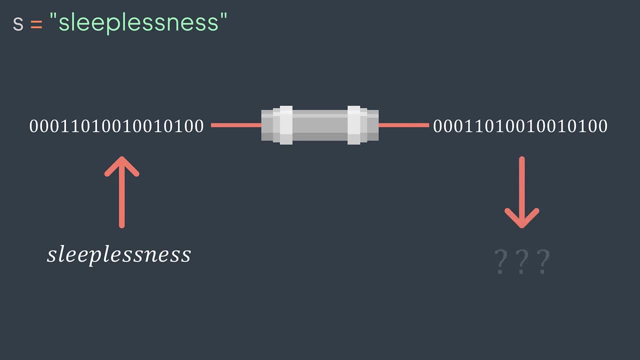 efficiently. but we should also know how to decode it to be able to read it. Here we had no problem to encode sleeplessness, But if we try to decode it we face ambiguity. For example, the first four bits are 0001.. Should they be decoded as SSS, As le LP? we 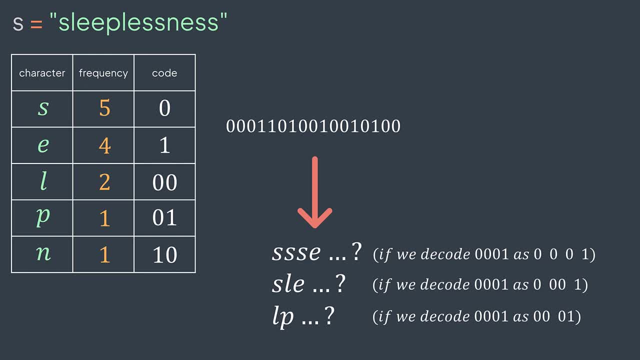 don't know. The reason behind it is that some codes are prefixes of other ones. Zero is a prefix of 0001.. And one is a prefix of one, zero. To visualize it, let's represent our code tree, where we write zero when we go to the left and one when we go to the right. 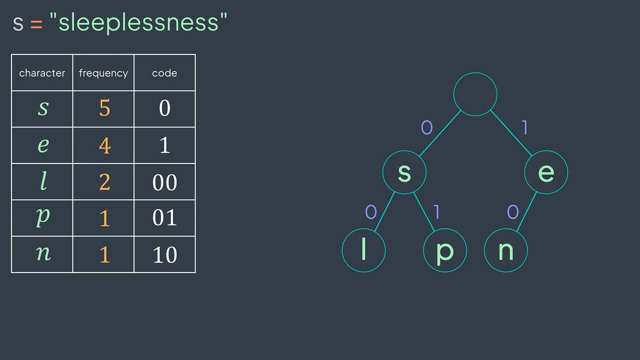 This is why we find, as when we go left l, when we go left left p, when we go left right, etc. We can see that some codes are prefixes of all the ones, because some character notes have children, which means that we take their code, you add something and we find another. 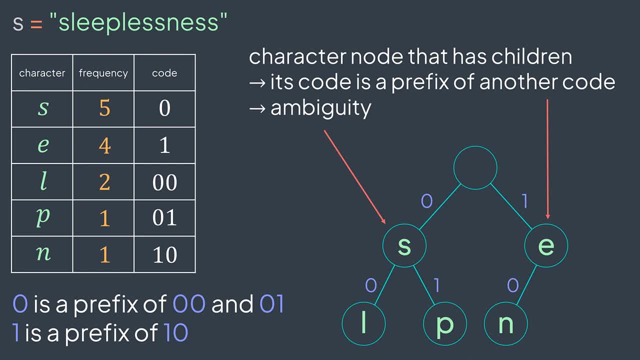 code. It's a prefix To avoid having. codes are prefixes of all the ones. All character notes have to beliefs. they must have no children bottom of the tree. By doing so we'll get what we call prefix free codes, no ambiguity. 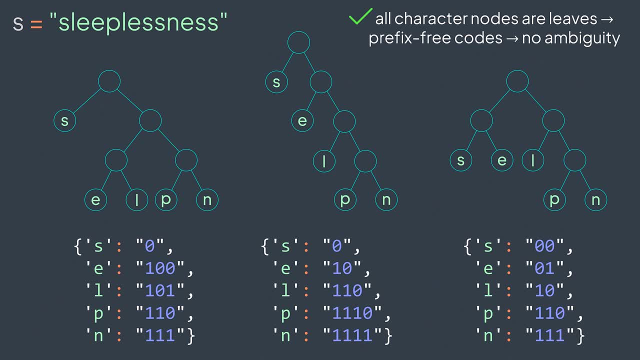 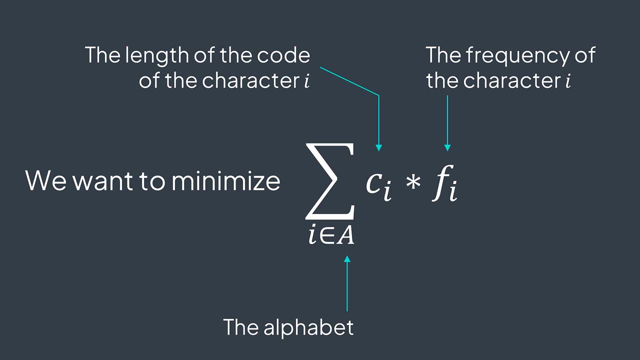 We have different valid trees that produce prefix tree codes, but how to build the most efficient one? By most efficient one we mean the one that minimizes as much as possible. the sum of ci times fi or I belongs to the alphabet, For example the alphabet of our. 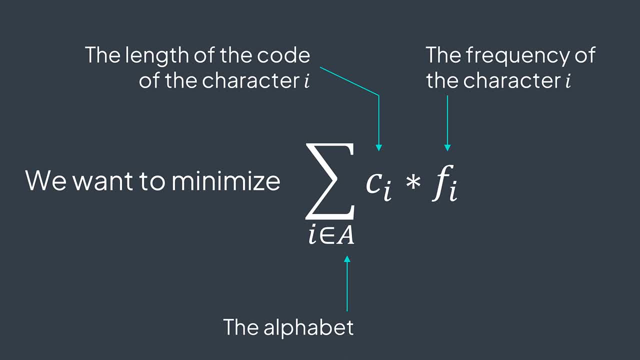 example, was SL EP n. Also, ci represents the code length of the character i and fi represents its frequency, Because this is what we want to minimize. in reality, this sum represents the required number of bits to encode our message And to calculate it for each character. 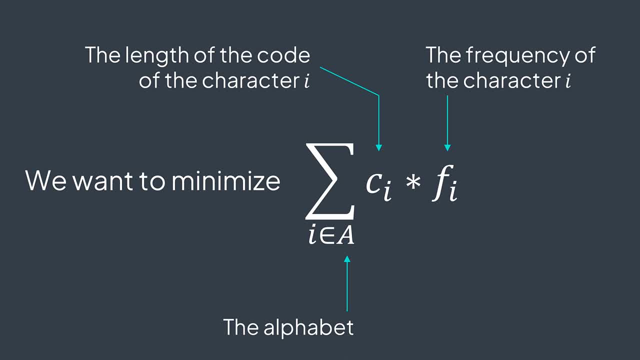 in the alphabet, we multiply the number of times it appears by the number of required bits to represent it. Well, to produce an optimal tree we're searching for, Huffman gave us an algorithm that we will see now. The example we'll work with is a part of the 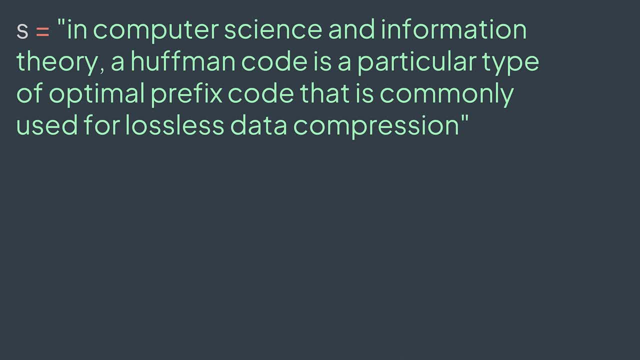 Wikipedia article on Huffman coding that you can read, obviously, for more information. First step: we count the number of occurrences of each character. This is what we find. Second step: we create a node for each character where we put the character and its frequency. 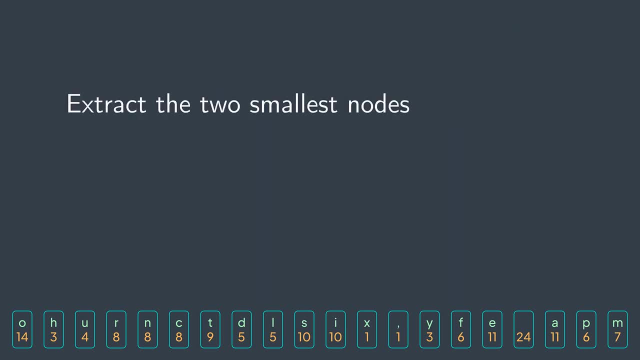 and we put them in a structure. And now we extract the two smallest nodes from the structure, we create a node that will be their parent, whose the frequency is the sum of their frequencies, and we insert it in the structure. By smallest we mean that have smallest frequency. We keep doing that until only one node remains in the structure, and then we put it in the structure. And now we extract the two smallest nodes from the structure. we create a node that will be their parent, whose the frequency is the sum of their frequencies, and we put 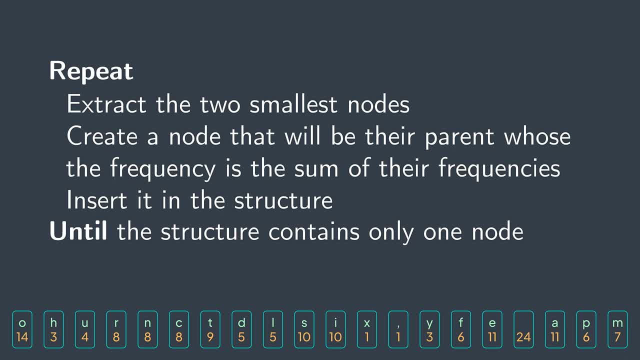 them in the structure. If we put it in the structure, it will represent our route, because we're building our tree in a bottom up way And Huffman algorithm is considered as agreed algorithm because at each iteration we do the greedy choice of taking the two smallest. 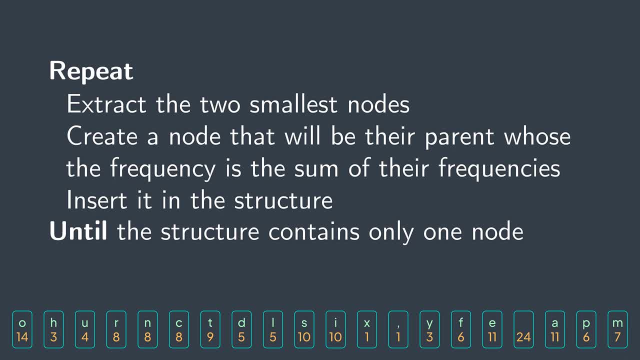 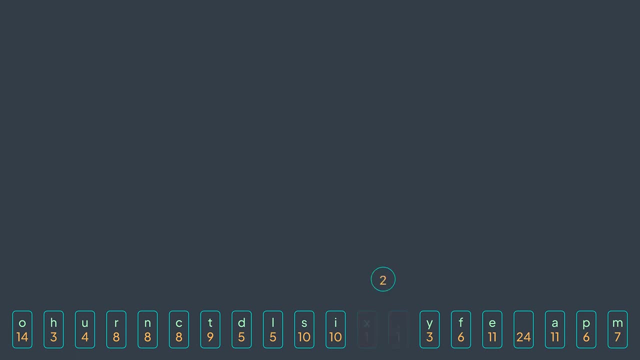 notes. Also, Huffman coding produces variable length codes. two symbols can have a different code length, not like an ASCII where all codes had eight bits. With this example, the two smallest nodes are X and the comma. We extract them, create to know that will be their parent. who is the frequency is the sum of their frequencies. 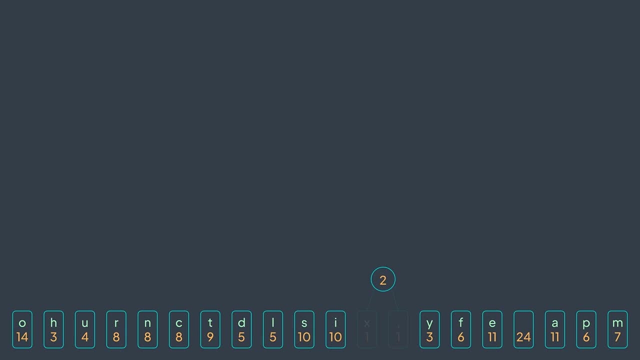 and inserted in the structure. Here we go to, because one plus one is to know that dark nodes are ones out of the structure, So we won't consider them when searching for the two smallest nodes. Next iteration: smallest nodes are the node we created now and the letter y. we combine them. 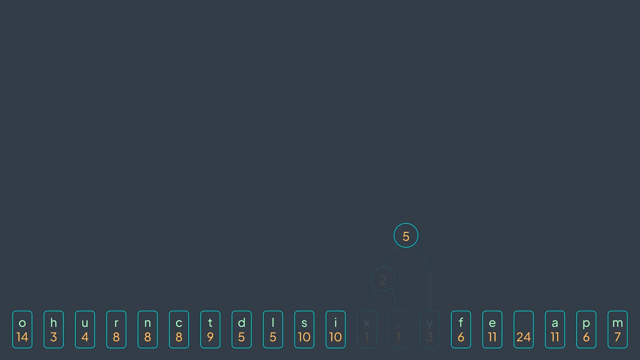 into a node whose the frequency is two plus three, five. Next iteration: the smallest nodes are the node age and the node. you will combine them with a node of frequency three plus 47.. Next iteration: D and L are the smallest ones. we combine them And we continue like that until only one node. 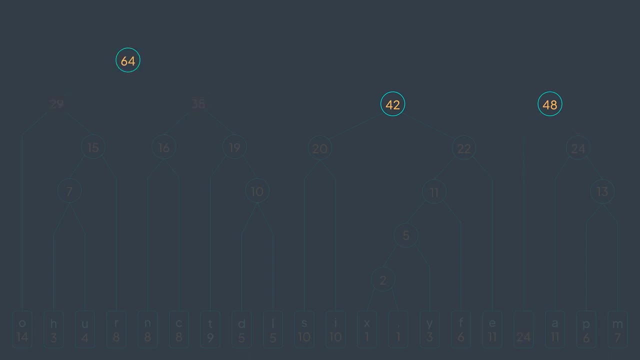 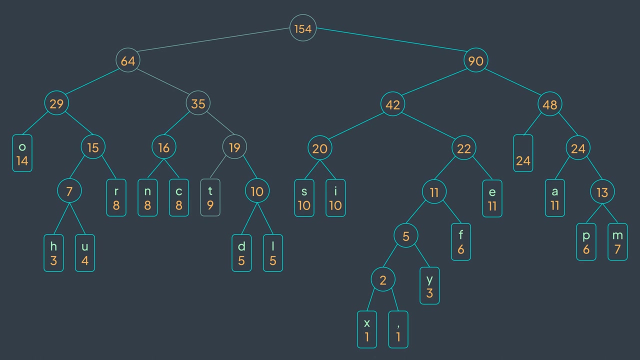 remains. That last node represents the root of our tree. we finished building it. Now you may be wondering why did we do that? I'll try to explain it. First of all, you need to understand that the depth of a character node represents the length of its code. 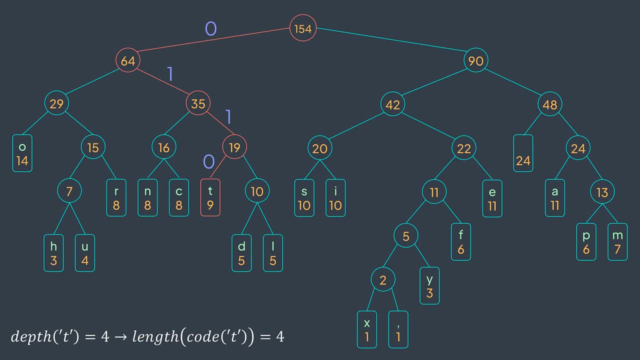 For example, he, the depth of T is four, So his code will have a length of four. it's 0110.. It's 0110.. Because we went left right, right left And we saw that we assign shorter codes for more frequent characters, But in sequence. 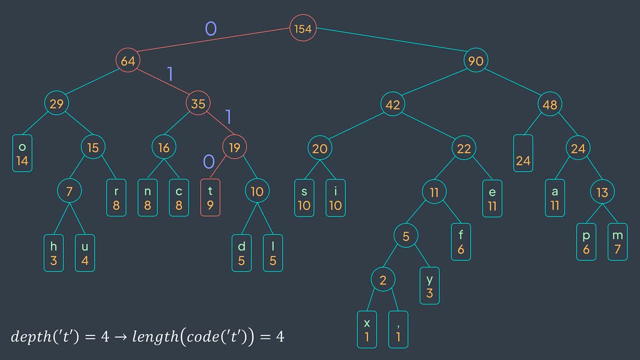 we assign longer codes for less frequent characters. This is why the deepest nodes represent the least frequent characters- x and the common, our example. the deeper we go in the tree while less frequent characters are, And it's the reason why we always combine the least frequent nodes, Because by doing so we take them. 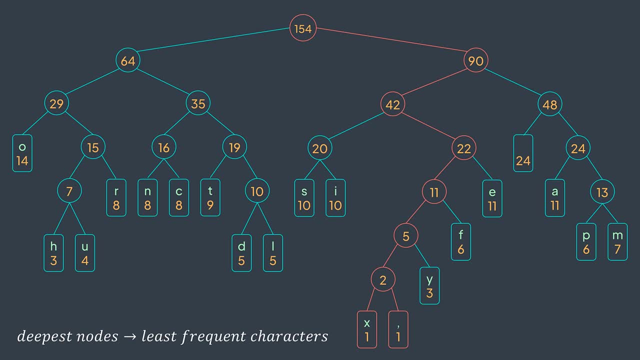 deeper in the tree. By consequence, more frequent nodes will be shrimpb Healing mixture later, So they will be on the first levels of the tree. they will be assigned shortcodes. For the formal proof will find a link in the description where you will see how we prove. 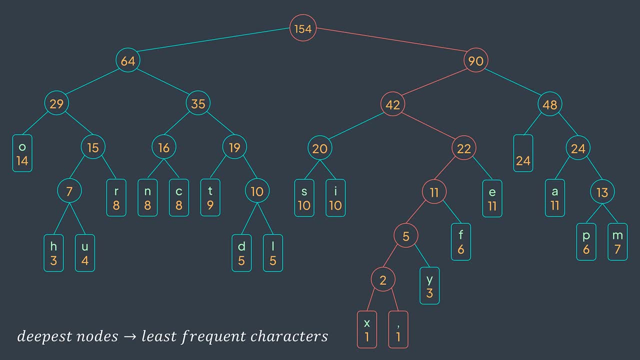 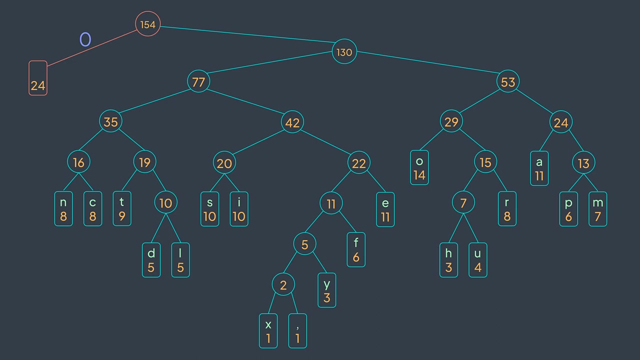 the optimality of half-mile algorithm by induction. Now, we doubt that. maybe in your mind is that here the space character is the most frequent character. Why did we give it a code of length three, 110, instead of a code of length one, zero, for example? Remember that we want prefix free codes, So if you 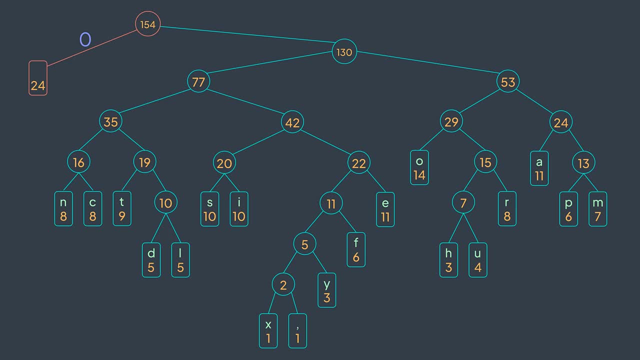 give the code zero to a character. all other codes must not start with zero. they have to start with one. in the tree, they must all be on the right side, which is not worth it. in this example, It's true that the space character is the most frequent one, but its frequency is smaller than 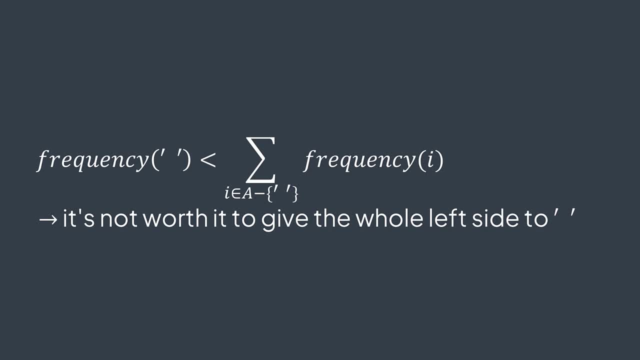 the sum of frequencies of all the characters. This is why at some point of the process, before the last iteration, it becomes one of the two smallest nodes that we combine, And combining means that we take those two nodes deeper in the tree. Therefore, the space character code will 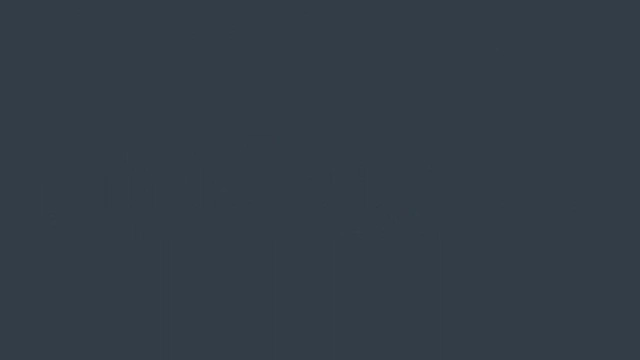 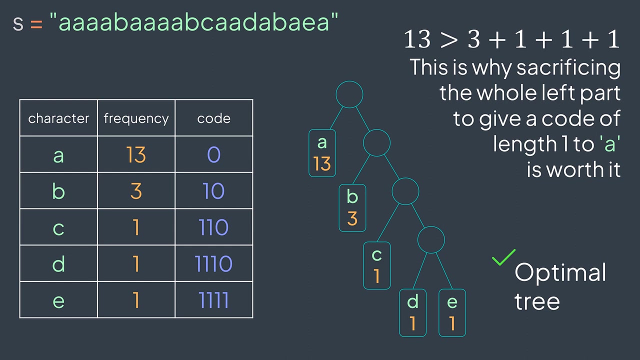 have more than one bit, But we can have examples where a character will have a code of length, one when its frequency is greater than the sum of all other frequencies, like here. Okay, now we build this tree, But what are we going to do? 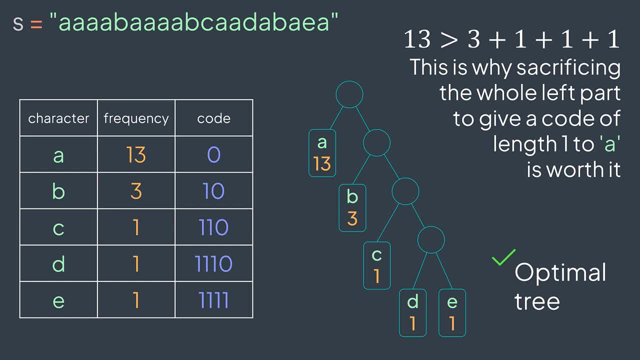 it. We're going to give it a code of length, one which is greater than the sum of all other frequencies, like here. Before answering, let's take a look at the implementation. First of all, we need to define a tree node. In our tree, a node can have a character. 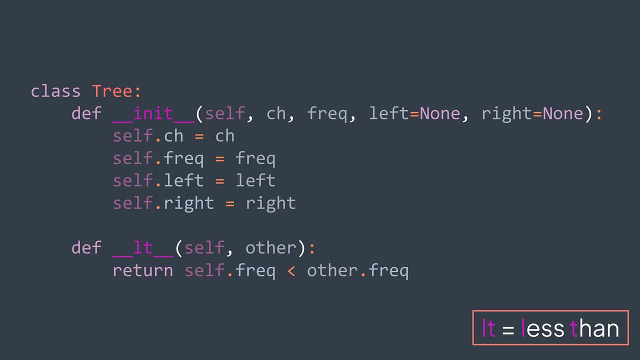 a frequency: a left child and the right child. Also, the order of our nodes is defined by the frequency. A less frequent node is considered smaller than a more frequent node. We mentioned this in our definition. Now in our build tree function. 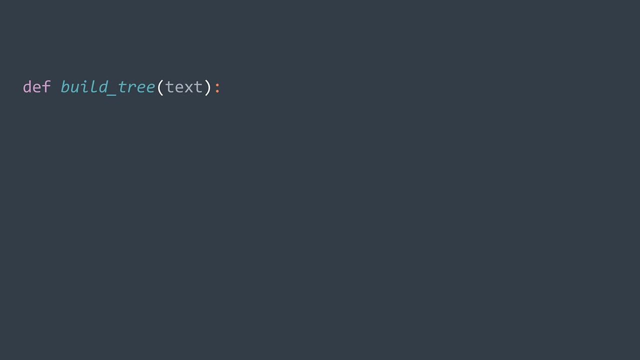 we start by counting the frequency of each character. For that we will use a hash table where the key is a character and the value is its number of occurrences. They all start at zero and increment at each character. We already have a class that does this in Python. 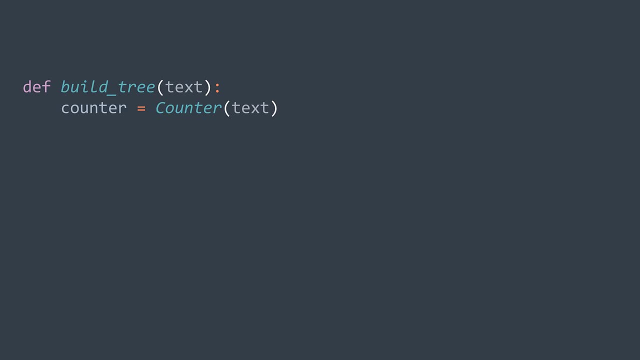 is the counter, but we import from collections module. we just pass our string as an argument when creating it and we got our hash table frequencies. Now we create a node for each character and we put them in a structure. But what structure we want to structure that allows? 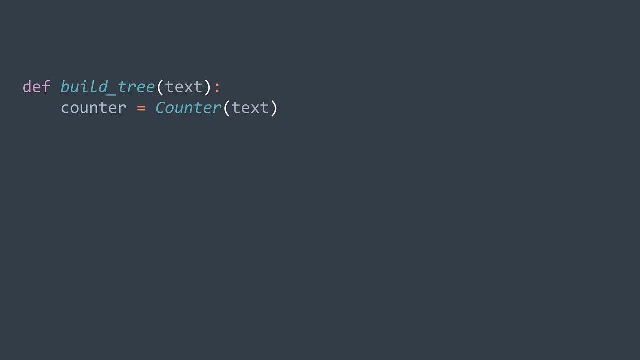 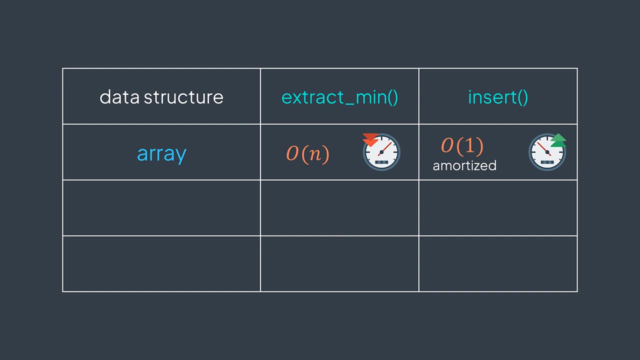 us to quickly extract the minimum element and insert an element. So that's what we're going to do. element. If we use an array, extracting main would cost all of n because we need to traverse the whole array to find the minimum- too slow. If we use a sorted array, extracting the menu would cost. 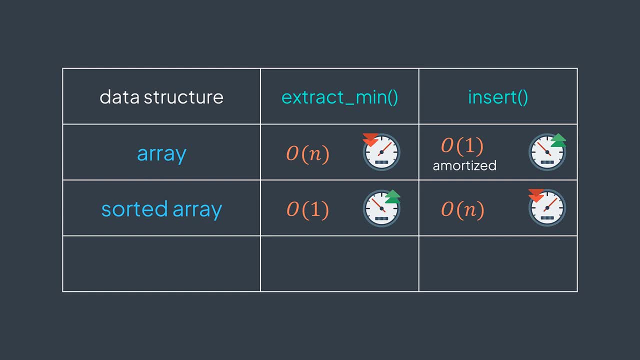 all of one because elements are sorted, But inserting would cost all of n because we need to maintain the element sorted- too slow. A very good choice to quickly perform these two operations is priority queue. extract. main and insert operations are both an off log n where n is. 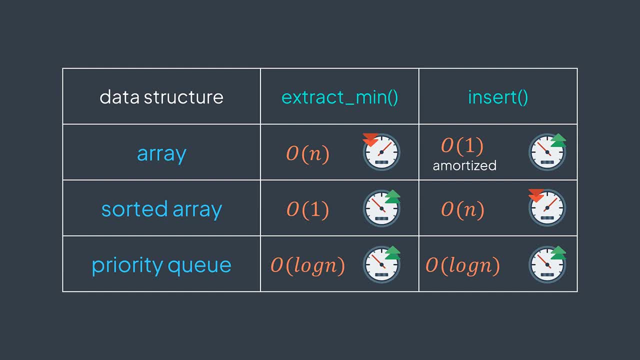 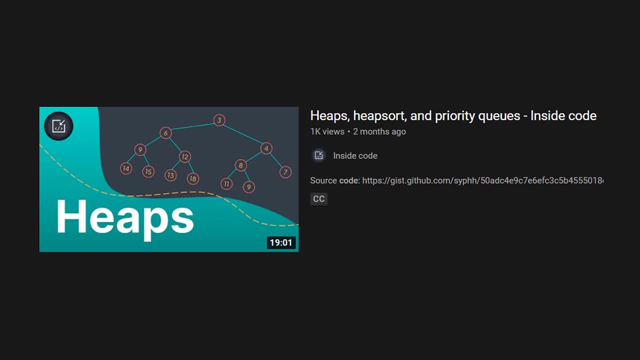 the number of elements. If you don't know what is a priority queue, I suggest you to watch this previous YouTube video I made. But, in brief, it's a queue, but where the next element to be popped is the minimum or the maximum, depending on our preference. Here we want it to be the minimum. 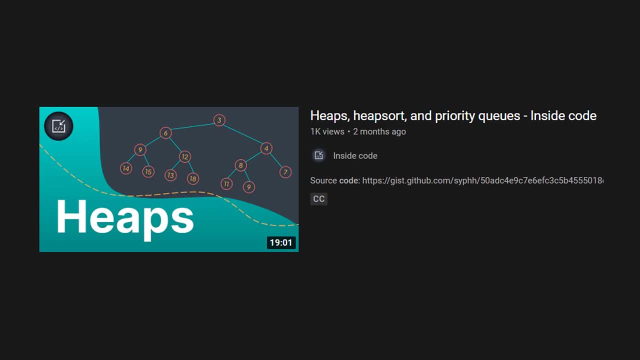 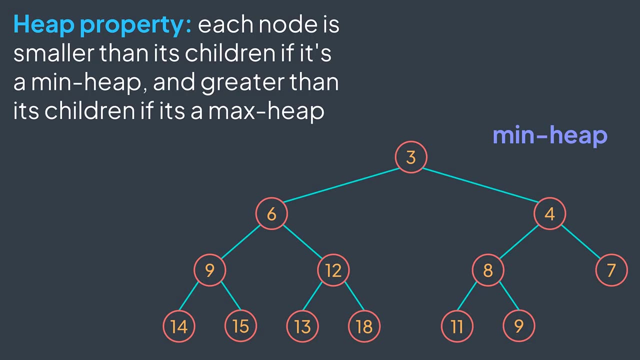 we want the smallest node. It's usually implemented with a heap and we can extract main and insert in a heap in off log n time the cost of maintaining the heap property, the property that says that each node is smaller than its children. In Python we can directly use the heap queue module without implementing a priority queue. 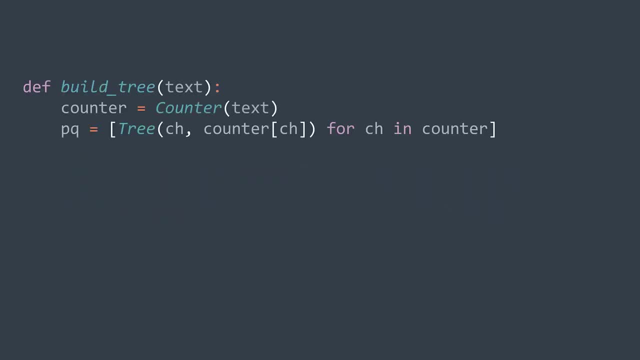 from scratch. So create an array that contains a tree node for each symbol present in the string. we are creating a node where the character is ch and the frequency is its frequency thought we can get from the hash map we built. Now we happy fight will convert it to a heap, And because we define the order of our notes, 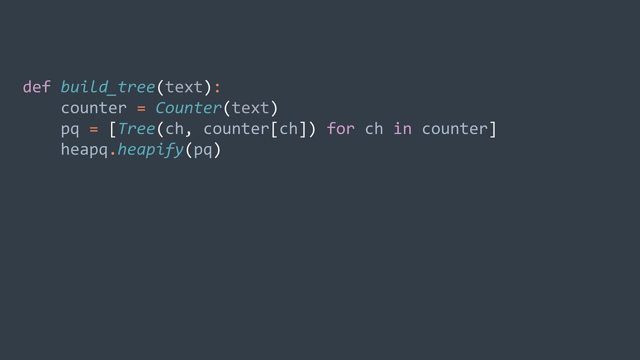 the function will be the same. We can also define the order of our nodes. The function will know that it has to order nodes according to the frequency, And now we saw that we keep repeating that process. we've seen, until we have only one remaining node, we write one length of. 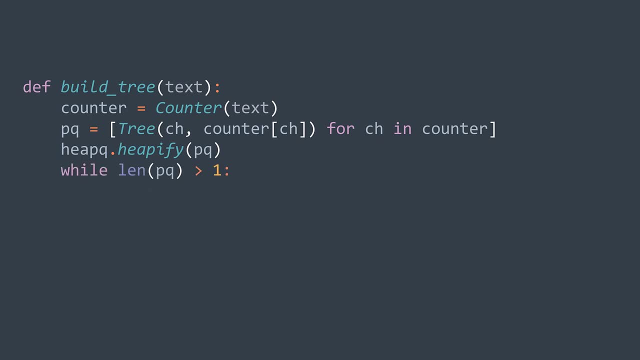 priority queue is greater than one. Inside the loop we extract min twice to get the two smallest nodes. then we create a node parent that has no character, who is the frequency is the sum of frequencies of the two nodes we extracted- holds the children of those two nodes. Last thing: 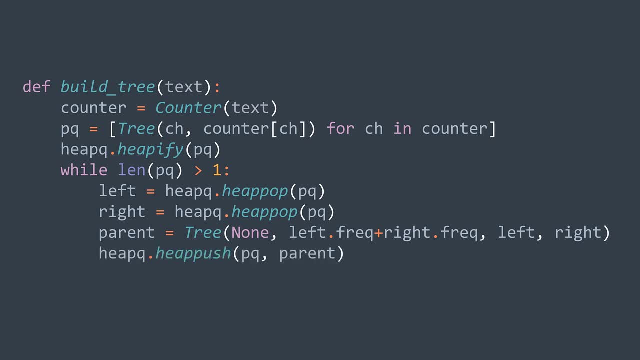 we just insert the node we've created now in the priority queue, As we were doing in the example. After the loop, only one node is remaining in the priority queue. it represents the root of the tree. we return it, So as output we'll get a node- the root, but that is connected to all the nodes we've seen before. 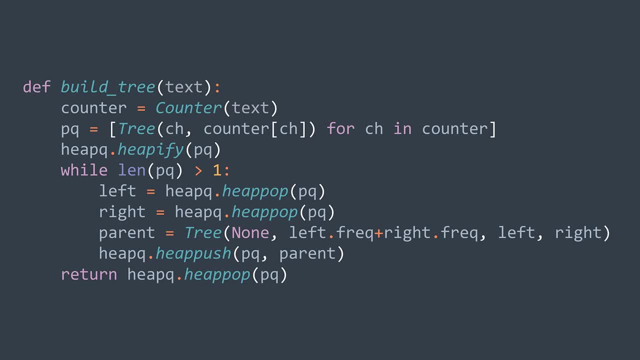 because we were putting links between the new node we create and the two nodes we extracted. Okay, now we know how to build the tree, what we will do with it. we first needed to build the encoding map, the one where we associate a code to each character. Remember that we were zero and 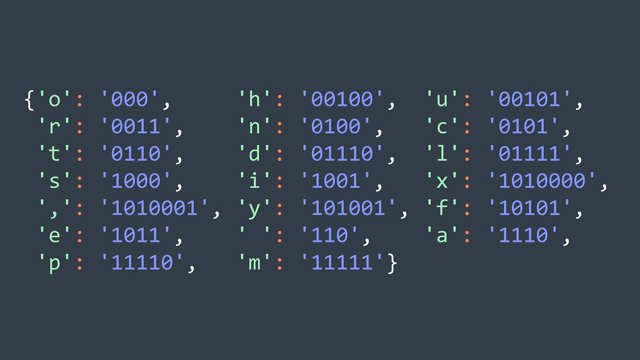 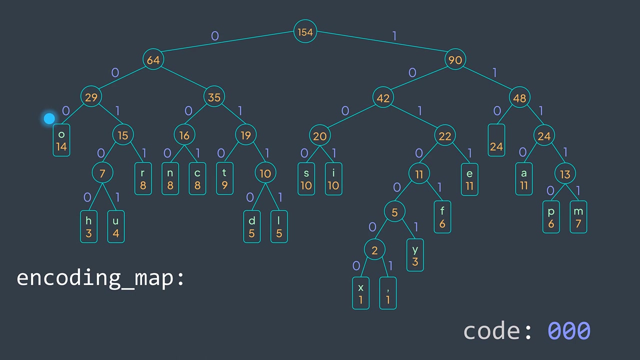 we'll go to the left and one when we go to the right. So we keep doing that with the depth first search traversal, And when we step on a character node, we assign the code we wrote to it With our previous example. we go left zero, left zero, left zero, and we found, Oh, so the code of the character. 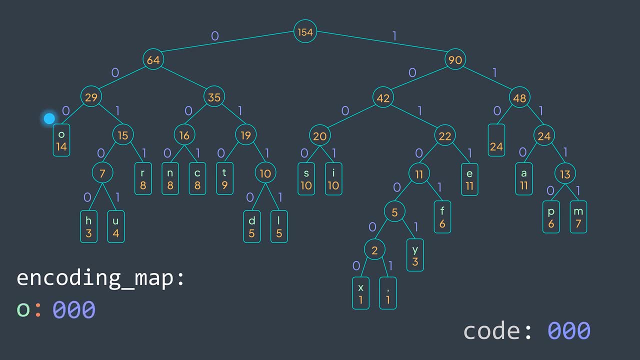 Oh is zero, zero, zero. Then we backtrack, we'll move a zero. we go to the right one, the left zero, the left zero, and we found another character, H. the code of H is 00100.. We pop and backtrack, we'll go to the right one and we find you the code of us 00101.. We pop and 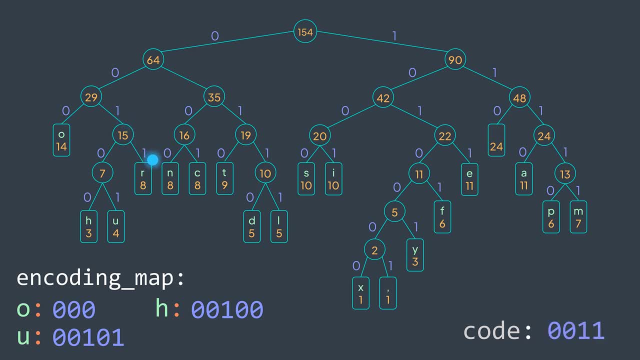 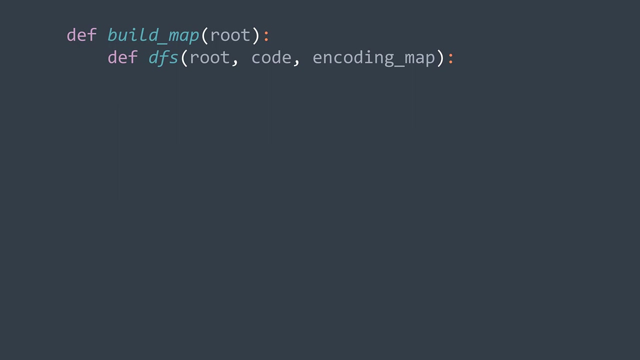 backtrack, we pop and backtrack. we'll go to the right one and we'll find our the code of our 0011. And the process continues like that until we finish. traversing the tree will get the encoding map In code as a parameter. we need the tree, then we need a DFS function. 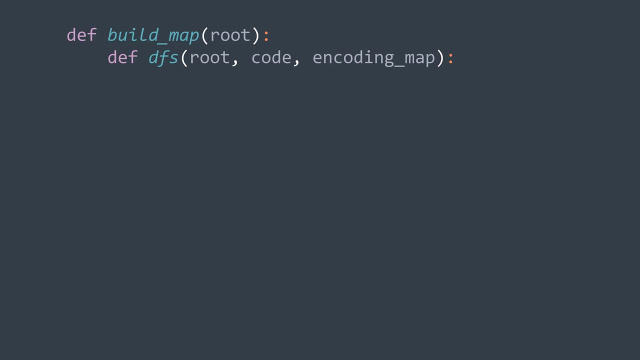 depth first search. It takes as parameter the actual node, the code we wrote until now and the encoding map. The base case occurs when we find the character node. If the character of the actual node exists, we assign the code we built to encoding map of root dot ch. We'll. 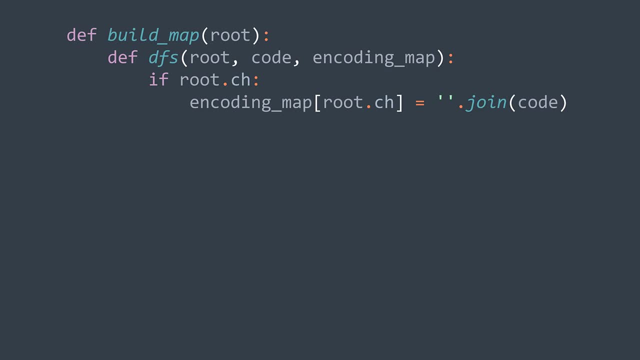 first join because the code is actually an array. we use an array to easily push and pop And in the recursive case we'll try both directions. left and right, we push a zero, we go to the left, then we pop the zero. when we backtrack, then we push a one, we go to. 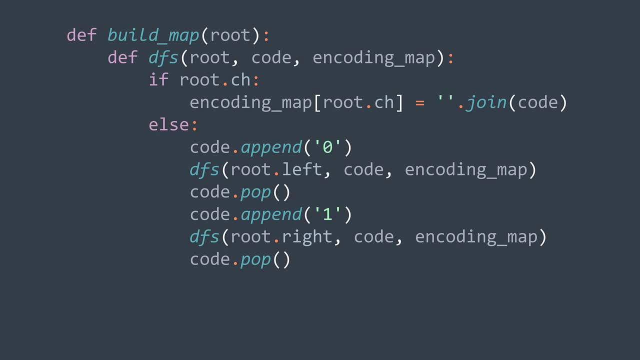 the right and we pop the one when we backtrack. We finished making our DFS function And in build map function we create the encoding map. we call the DFS function to fill it. the code starts as an empty array and we return the map. Now we have our tree and our 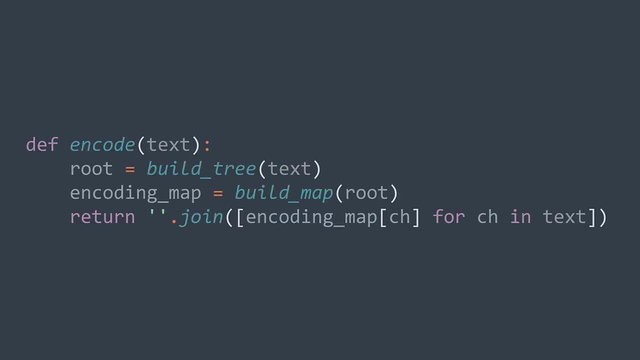 encoding map we can encode and decode. To encode very easy: Once we have our encoding map, we just replace each character in the string by its code. We'll put encoding map of ch for each ch in text and we join And. 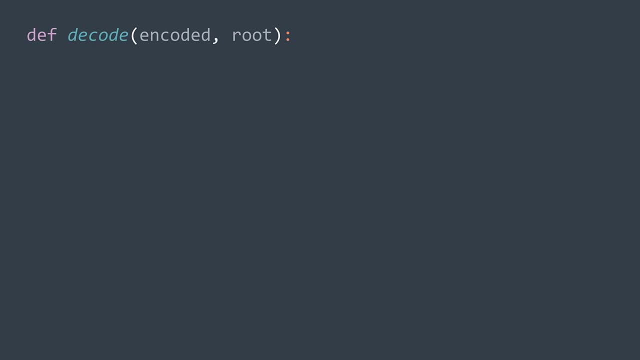 for decoding. we need the tree only. Our encoded string now contains zeros and ones only. The idea is that we start from the root of the tree, we go to the left if we read a zero, we go to the right if we read one, And if we step on a character node, it means that 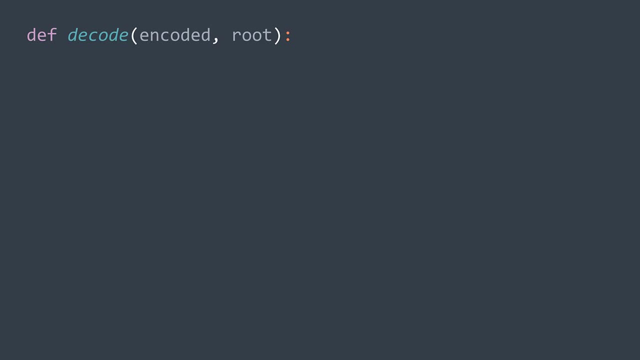 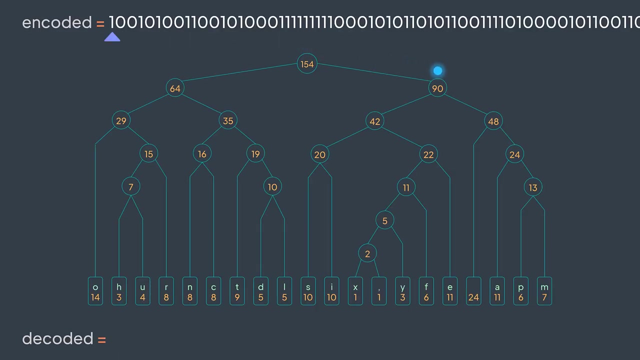 the code you read now corresponds to it. We write it. and to decode the next character With our previous example, we start from the root. we have one, so we go to the right. then we have zero, so we go to the left than zero, so we go to the left. 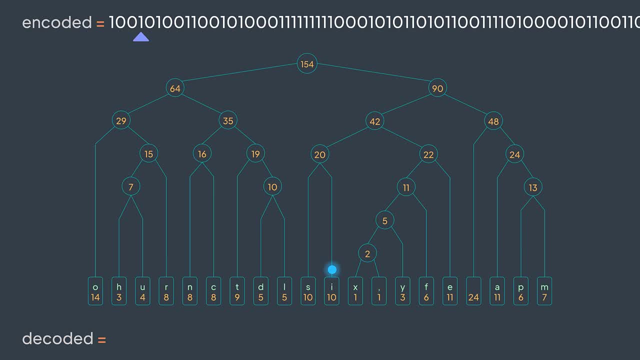 then one, so to the right. And here we found a character. note the character I added to our decoded string. and we go back to the root. Now we have zero, so we go to the left than once we go to the right, then zero to the left than zero to the left. And we found the character and we added: 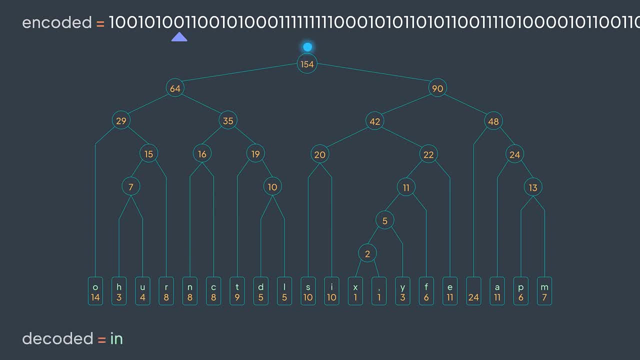 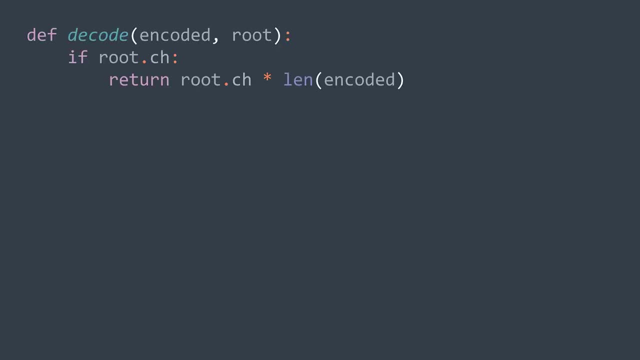 to decode it and we go back to the route as the process continues like that until we finish traversing encoded. encode refers have early exit condition: If the route has a character that the whole string is made of one character. we just repeated length of encoded times. If it's not the 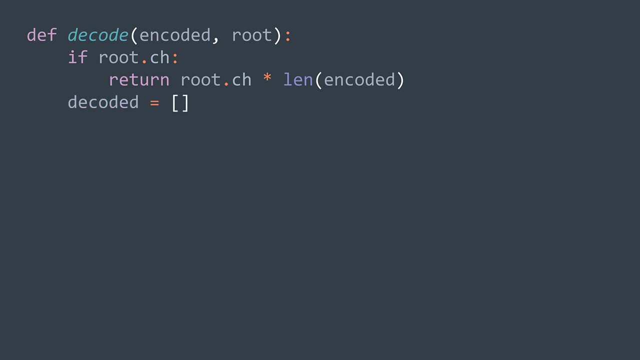 case we create an array decoded where we will put our decoded text. we put a note on the route and restart for each bid and encode it. If it's zero, we take him out to the left, else off into 1. 00. if it's a 1. 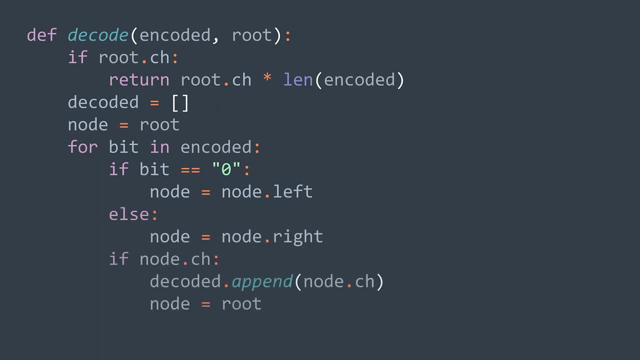 00. if it's 0, take no to the right Now. if not that ch exists, we add it to the coded and we take no to root again. That's it. We've been able to know that it's the right character because our codes are. 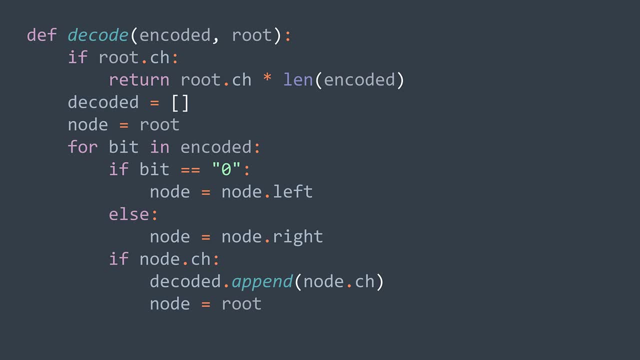 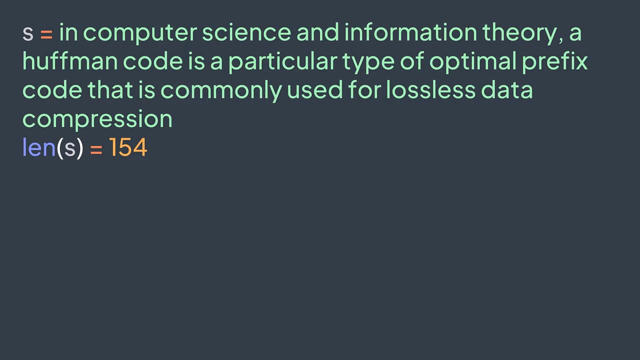 prefix free. There is no ambiguity here. After the loop, we just joined the coded characters and we return. And now we know how to encode and decode tax with half man coding. Let's measure its efficiency with our example. The length of our example string is 154 multiplied by eight. we got 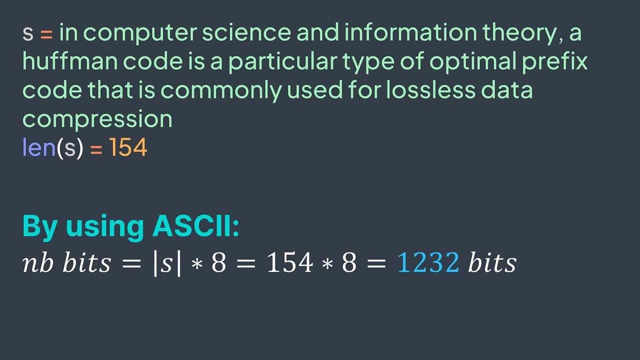 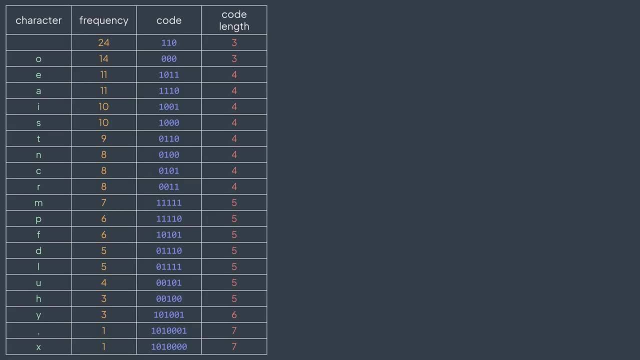 1232 bits. we need 1232 bits to store it. if we use ASCII encoding With half man coding, in this table we have the character, it's frequency, it's code and the length of it code. We said that the number of 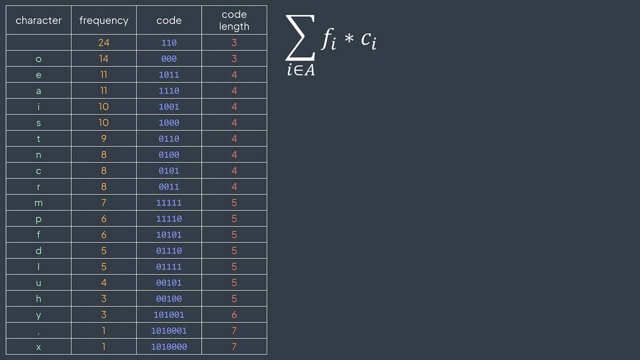 required bits is the sum of the frequency times, the codeline for each character. So we have 24 times three plus 14 times three plus four times three plus four times three plus 14 times three plus 11 times four, and so on. We got a total of 626 bits, way less than 1000 and 232.. But 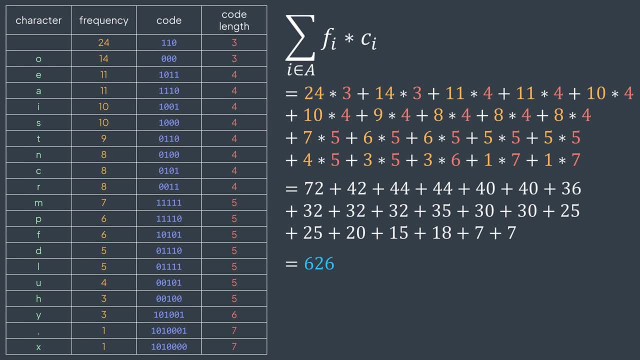 we don't forget that we will also need to store the tree and the encoding map to be able to encode and decode, Because if we store the encoded message without history, we won't be able to decode it, And so on. these additional structures cost space. This is why we have 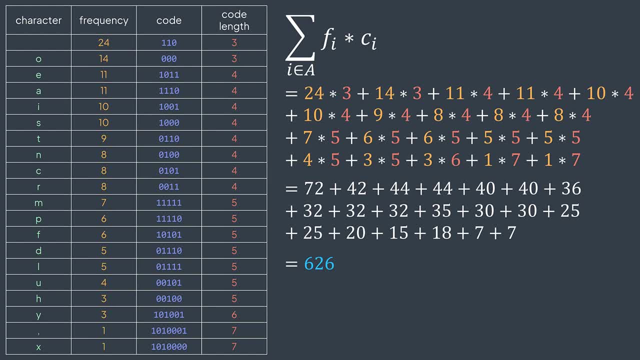 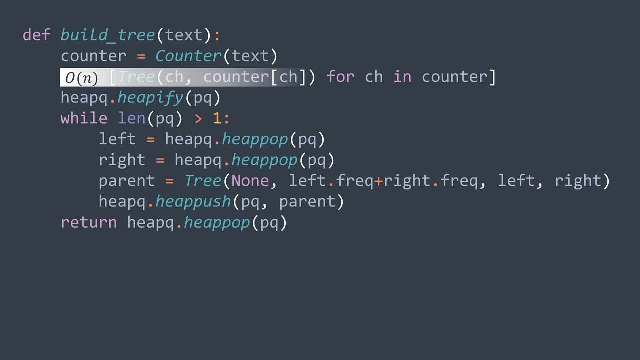 to do it as efficiently as possible For the time. complexity. if we don't count the cost of counting the frequencies, we have O of N for creating the N initial nodes. where N is the number of symbols will also have O of N for heapifying. We've seen why the 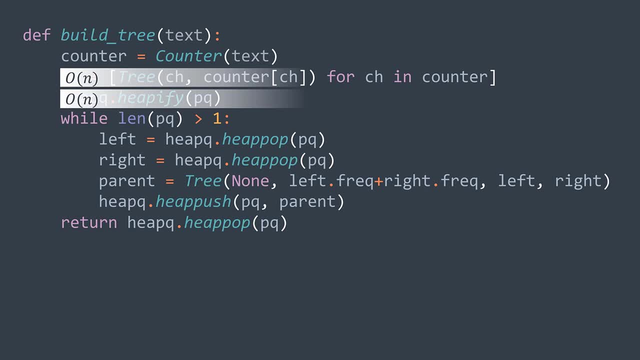 cost of heapifying is of an in the heaps video. And now for the loop. at each iteration we're extracting two nodes and inserting one node, so the size decreases by one. We initially have n nodes and we stop when we have only one node left. 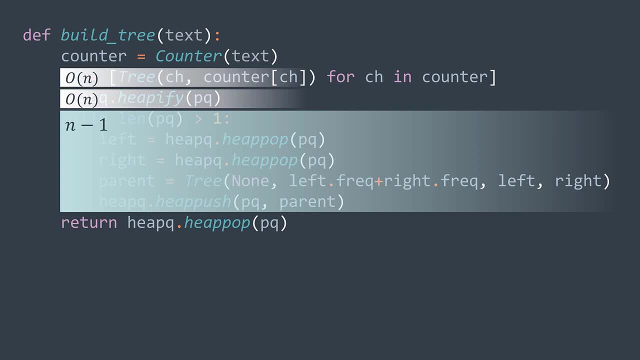 So we'll have N nodes and we stop when we have only one node left. So we'll have n nodes and we stop minus one iterations. We're using a priority queue and extracting bin and inserting in a priority queue. cost of log n. In total we have of m plus of n plus n minus one times of log n. 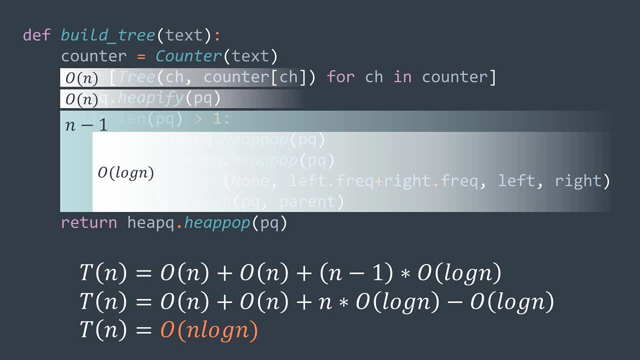 we'll get an O of n log n time complexity, where n is the number of symbols. We also have an O of n time solution if we're given frequencies that are already sorted And we finished learning about how Huffman coding books. The astonishing thing is that. 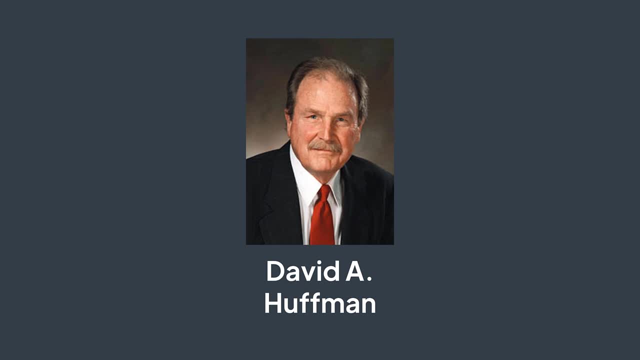 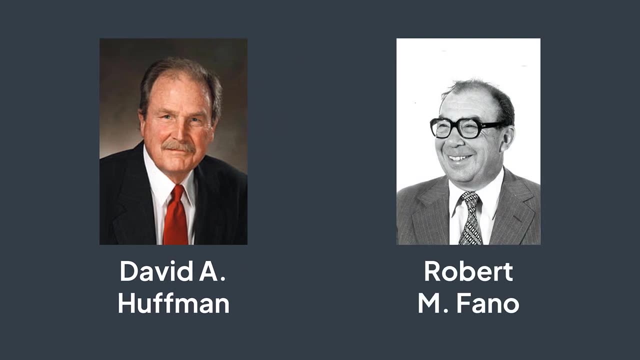 David a Huffman developed this algorithm while he was still a student. It was a term paper for his information theory class. His professor was Robert M Fano, the person who, with Claude Shannon, developed Shannon Fano coding another code similar to, but slightly less efficient than Huffman. 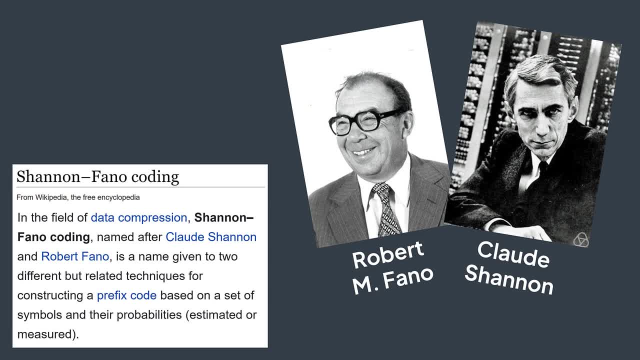 coding, The student surpasses the master. We reached the end of this video. I hope that now you understand how Huffman coding works. Like and subscribe if you enjoyed, and see you in the next one.